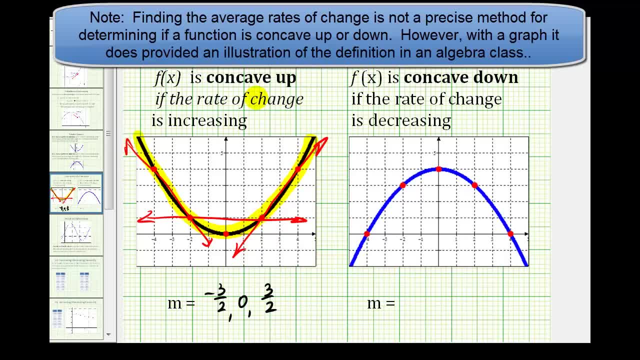 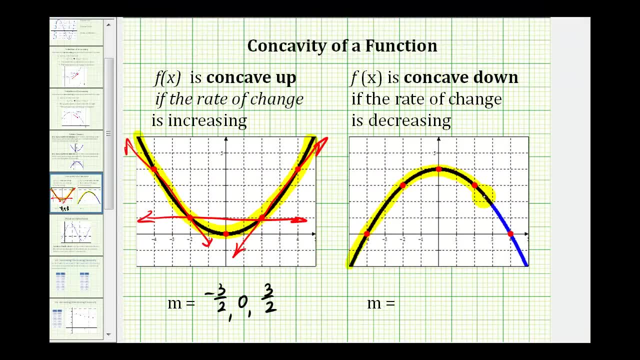 are increasing and the function is concave up. Similarly, a function that's concave down will have a shape like this that looks like an upside down cup that would not hold water. But, again more formally, a function is concave down if the rate of change is decreasing. 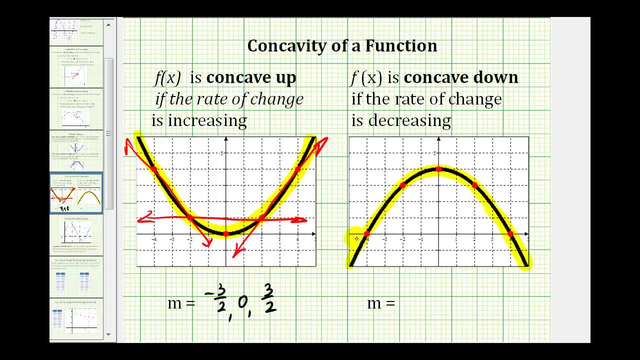 And then again, if we did the same thing and found the average rates of change through these two points, these two points and these two points, the slopes of these lines would be positive three-halves zero and negative three-halves. 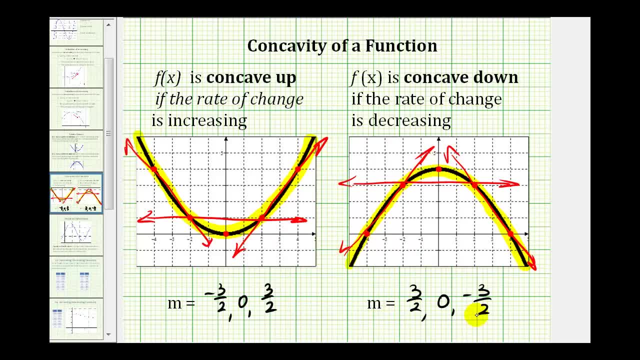 And notice now the average rates of change are decreasing And the function is concave down. And then where a function changes concavity, we have a point of inflection. So let's go back to our problem. If we take a look at the left side of this graph, 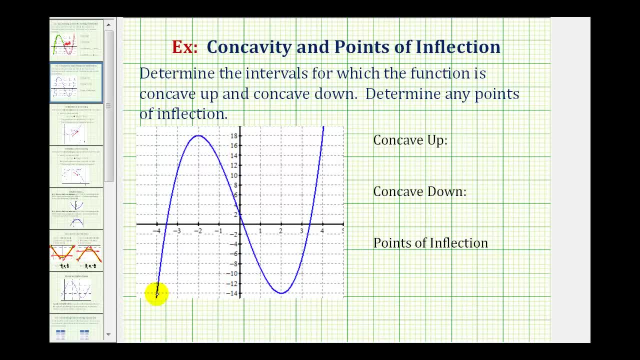 notice how it looks like it would form an upside down cup And therefore the left side is concave down And then somewhere near the y-axis looks like right on the y-axis it changes from concave down back to concave up. 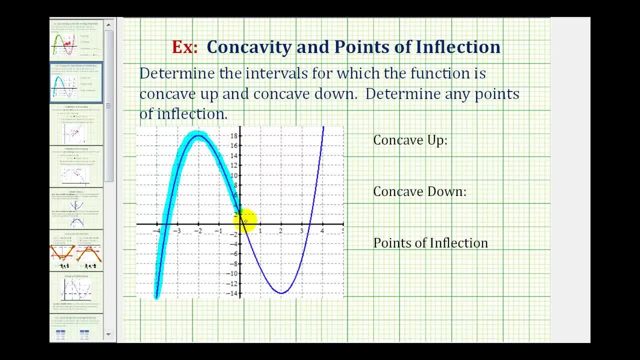 Notice how the graph would form an upward facing cup. So on the right here the function is concave up And, as I mentioned, it looks like it changes concavity right at the y-axis And this point here would have coordinates zero, comma two. 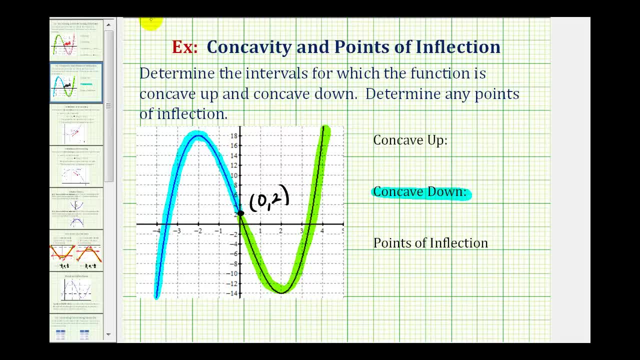 So the left piece or the blue piece is concave down And the green piece or the right piece is concave up. So the function is concave down from negative infinity to zero, Or for what we could say when x is less than zero. 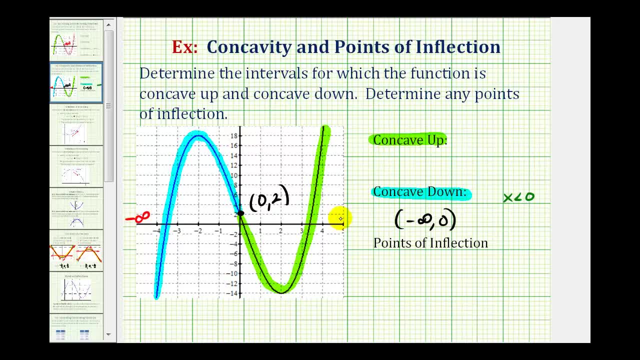 And the function is concave up from zero to positive infinity. Or we could say: when x is greater than zero, We don't include zero in the interval, because that's where it changes concavity And that's why the point zero two.